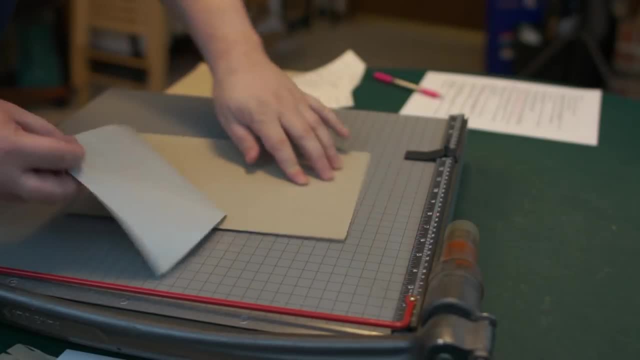 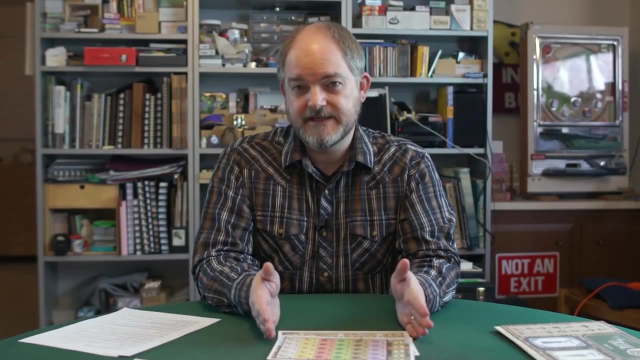 stick down the sticky part and then peel off the rest of your labels. That'll make sure you get your labels stuck on exactly where you want them. Now I left the labels and the cardstock untrimmed when I stuck these together so that I could make one cut and clean it up at the very end. 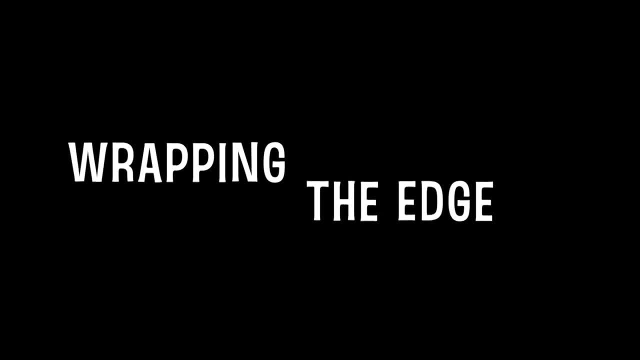 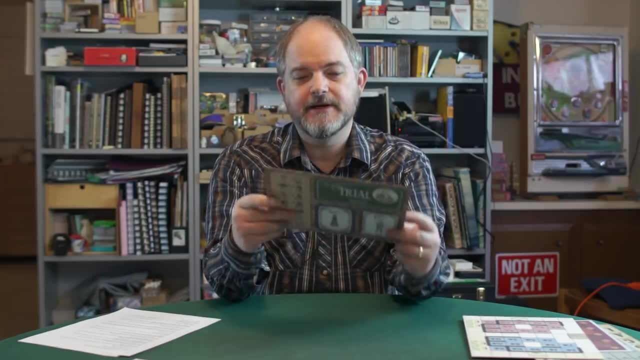 For a slightly prettier edge, you can wrap the label around the cardstock. So I'm still doing labels on cardstock here, but in this case I'm wrapping the label around to the back so that the edge has color and not just plain white. For this cardstock I'm using some artist's 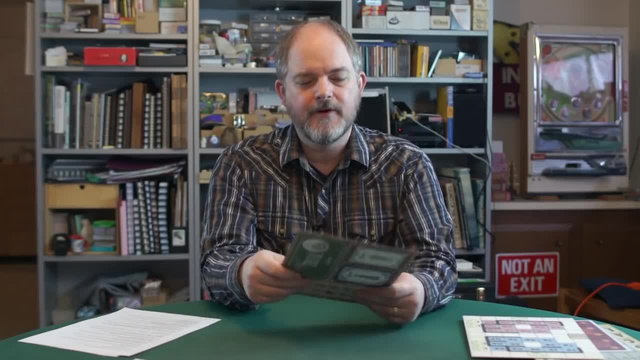 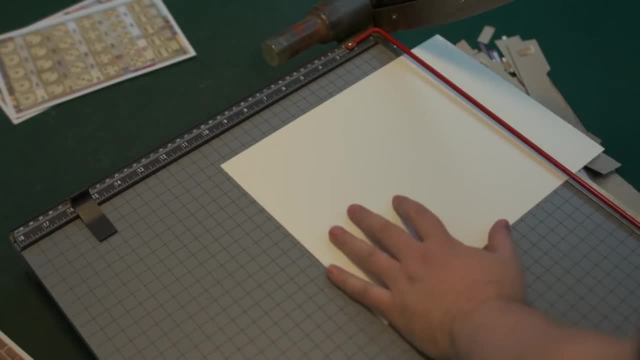 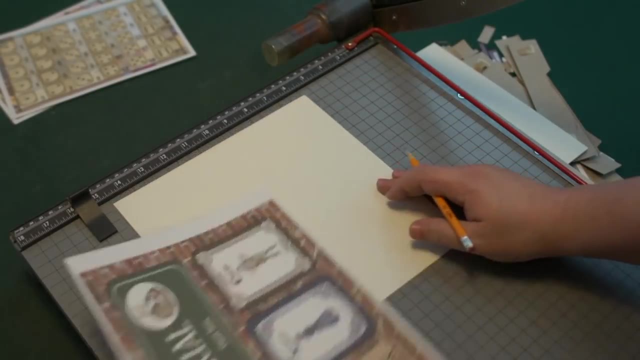 drawing paper, which is still a little heavier than that chipboard from the cereal box In this case. I'm trimming down this second piece of cardboard and I'm going to use my blank line for my cardstock, the core. I'm trimming the cardstock to the right size of the finished board, but I'm still leaving. 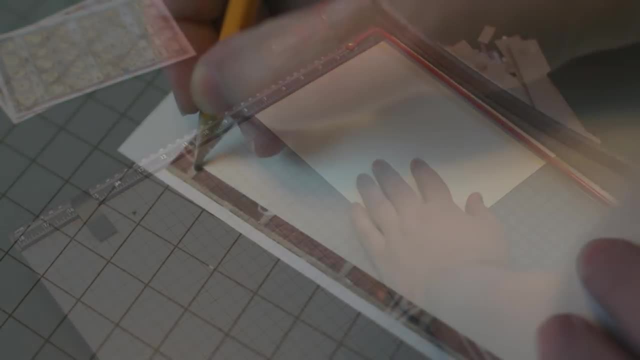 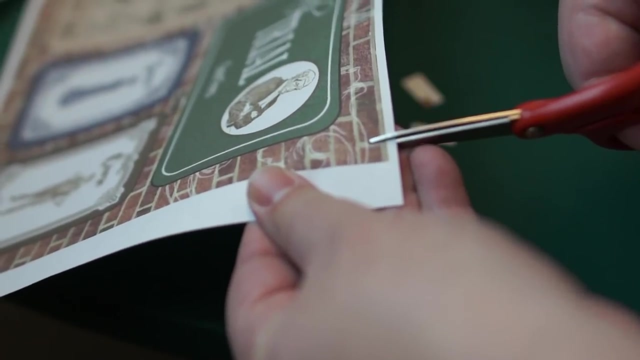 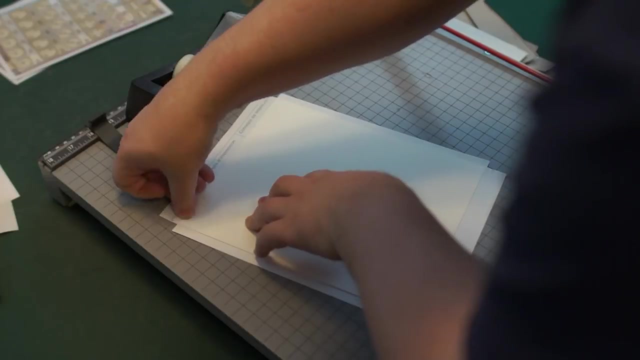 the label big. I'm going to mark the corners of the board on the label. I'm going to cut in at those corners a little bit wider than 90 degrees and then I'll have tabs basically that wrap around the edges of that core and give me a nice clean edge all the way around the board. Here I'm using 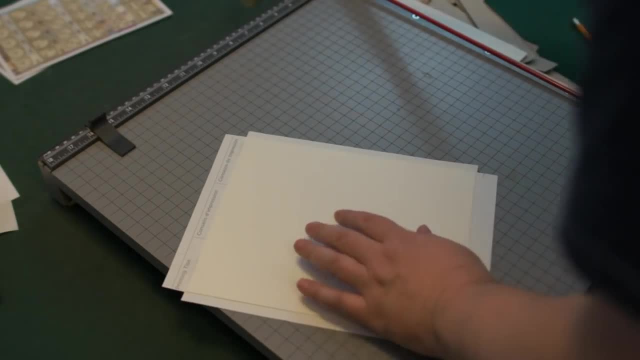 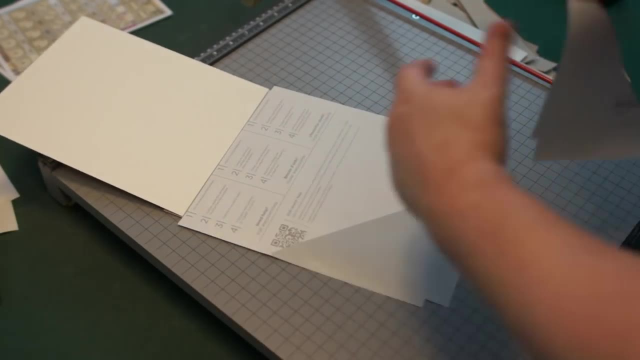 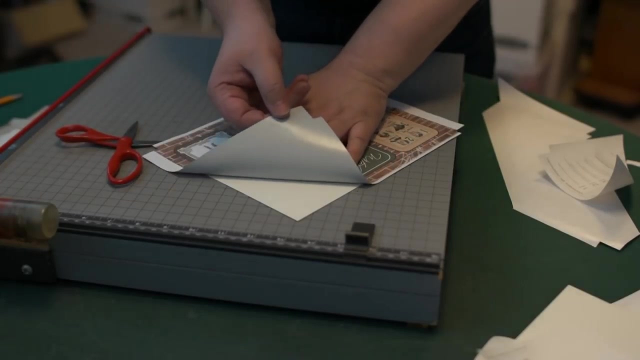 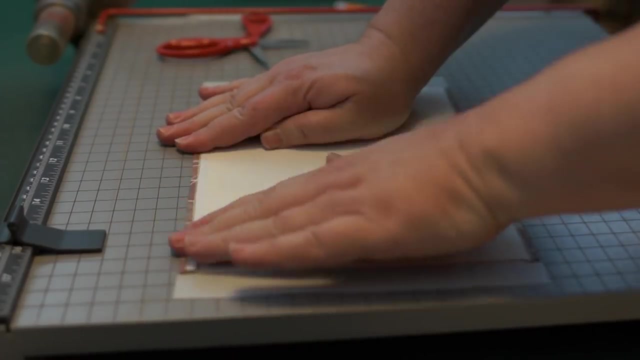 a piece of scotch tape to clamp the label to the core so that it doesn't slide around while I'm peeling off the backing sheet. This technique is actually kind of fun and it gives you a better looking edge than just trimming it out. 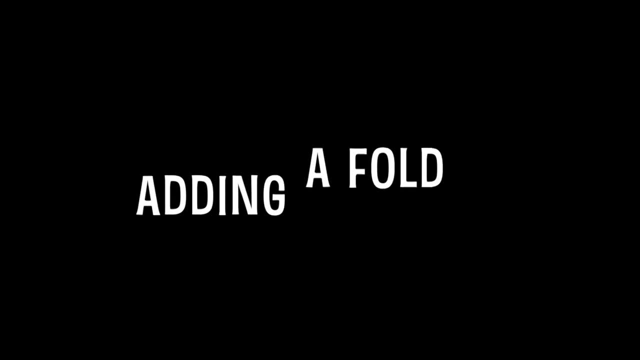 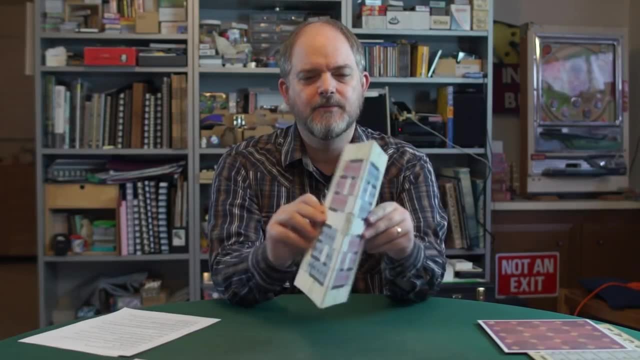 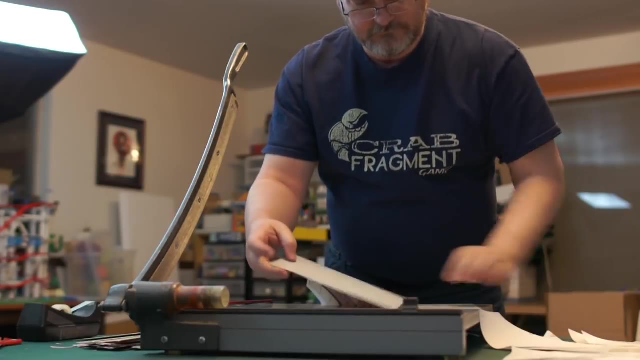 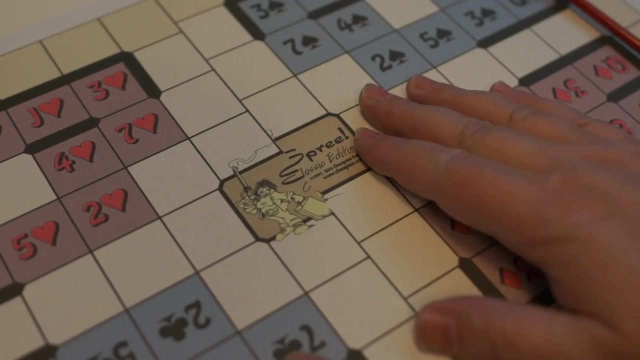 This spree board is two pages, and so we're going to print each one separately and then we're going to connect them using packing tape. on the back. Again, I only cut when I have to, so the outside edges I'm leaving raw, but I'm cutting the clean line down the middle so that I can line up these two pages. 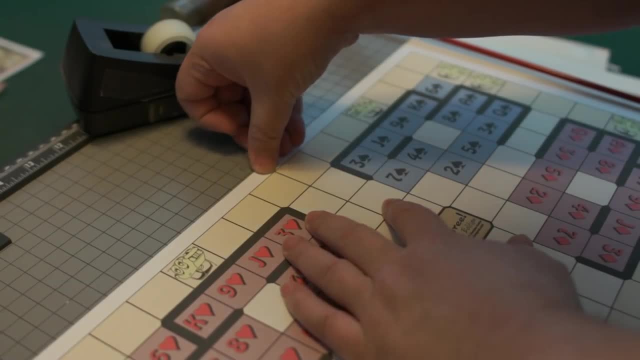 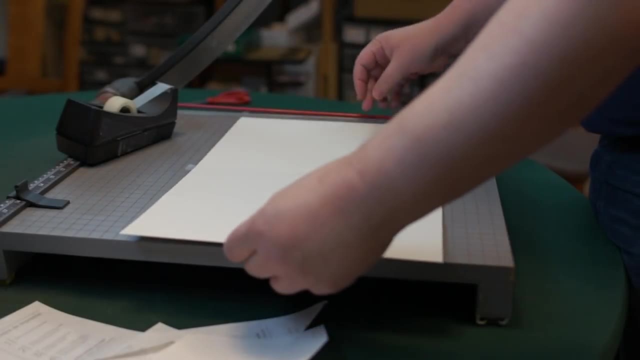 I'm connecting them on the front with a little bit of scotch tape. I'm going to take that back off after I've got the hinge built, but I just use the scotch tape to keep the pieces together. I'm using three strips of packing tape for this hinge. 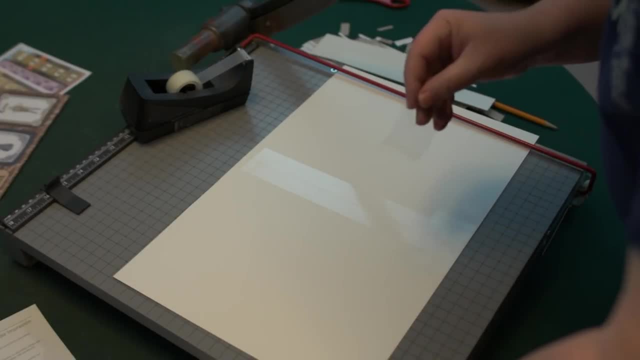 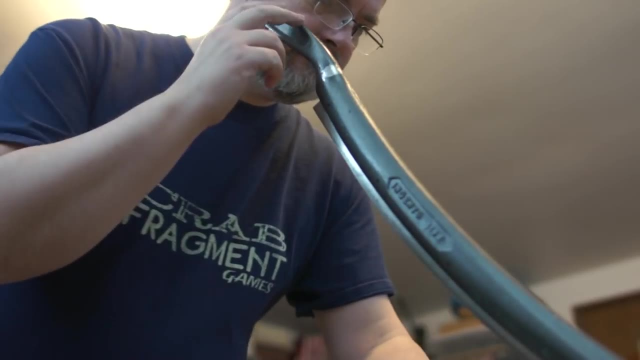 I use one long piece for the hinge itself and then I reinforce it at both ends with another short piece that goes across. Now the board's all taped together, I'm going to trim the outside edge so that it's a nice clean line all the way around. 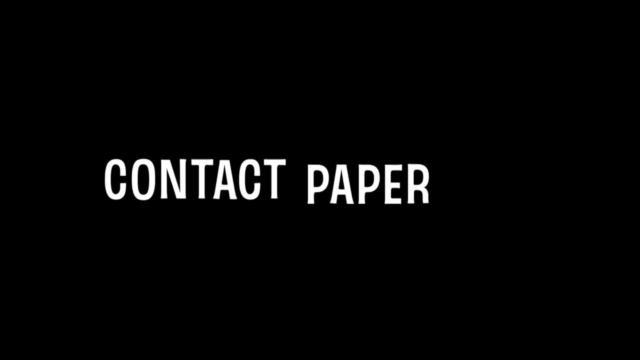 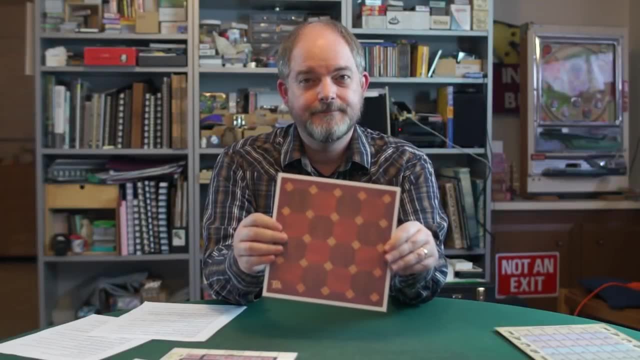 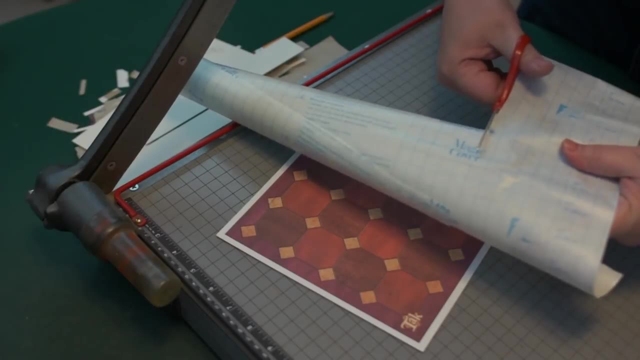 If you want a board that's a little more durable, you can cover it with contact paper. That's what I've done with this one piece tack board. Contact paper is adhesive paper. it's for protecting drawers or cabinets, and the kind that I'm using is perfectly clear, but it does have a gridded backing. 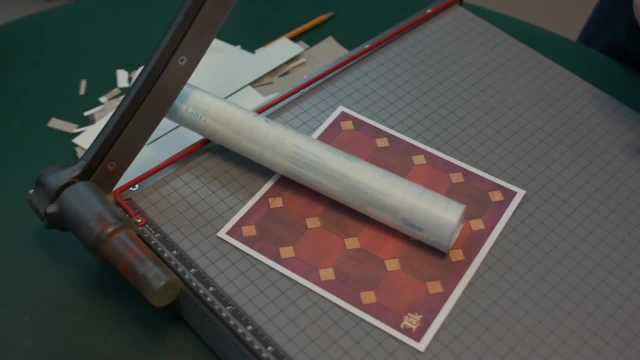 sheet so I can cut it straight and get it the right size. I taped this piece of contact paper to my work surface because it keeps curling up and going all the way down. In fact, this piece was in the room. probably the people that did allemaal. 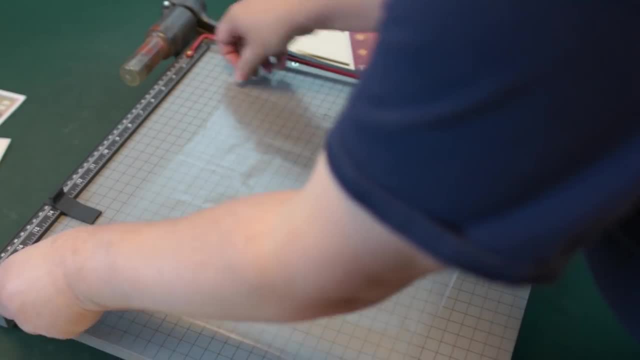 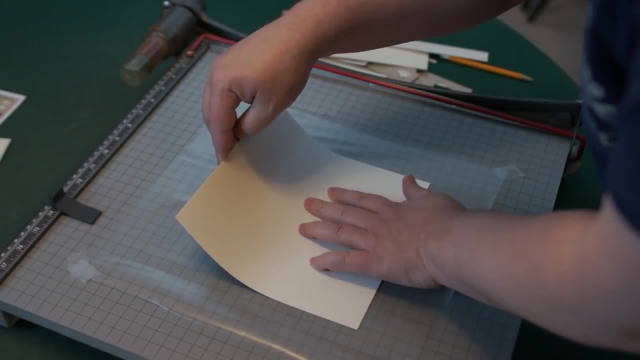 going crazy on me, so I taped the corners down so it wouldn't get away from me. I'm putting down the board one edge first and then I'm gonna curl it slightly so I can press as much air out of there as I can. 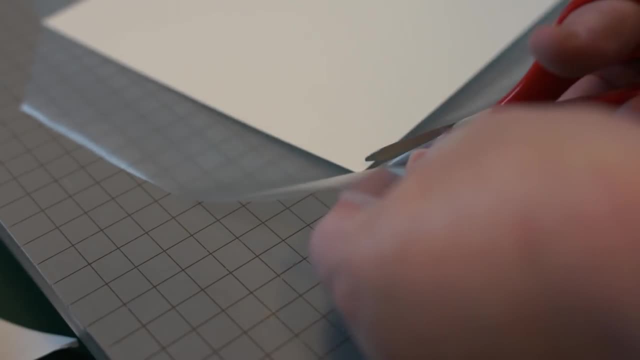 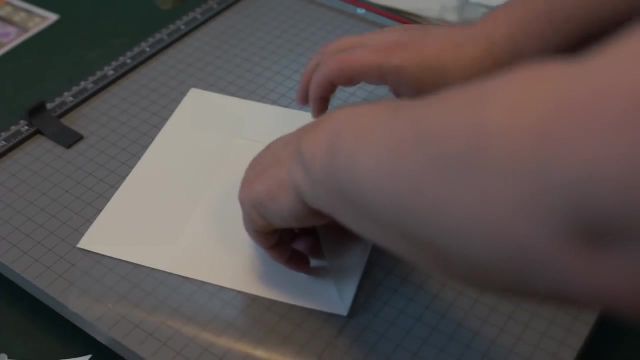 Just like with the label, I'm gonna trim these corners out to a little wider than 90 degrees so that when they wrap around they won't interfere with each other. Then wrap the edges nice and tight and you've got yourself a nice covered board. 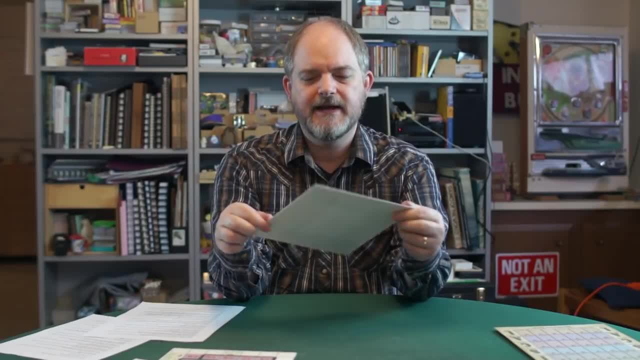 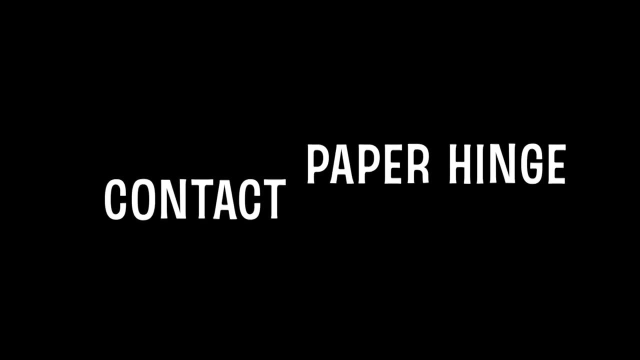 This is not 100% waterproof. Water can still get in the corners and on the back, obviously, but it'll certainly stand up to a lot of spills, a lot more abuse than just the printed paper would On this Jacob Marley board. I wanted to fold it in half. 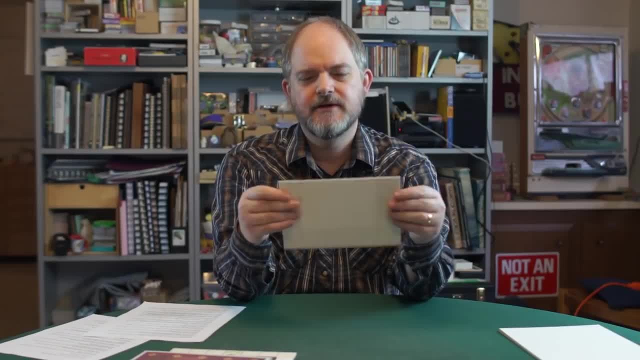 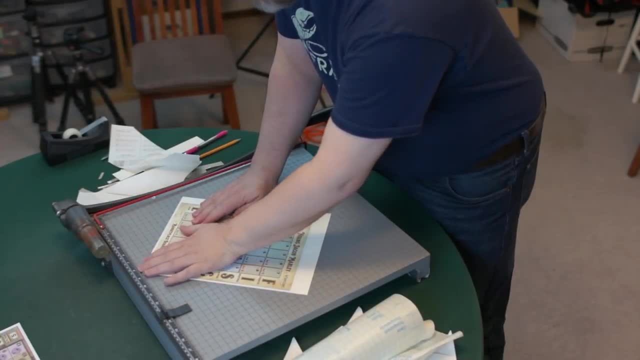 I'm gonna use the contact paper on the front to form the hinge that keeps the thing together in the box. This Jacob Marley board is a single sheet to start with. I'm gonna trim the edges and then find the center And once again I'm cutting a sheet of contact paper. 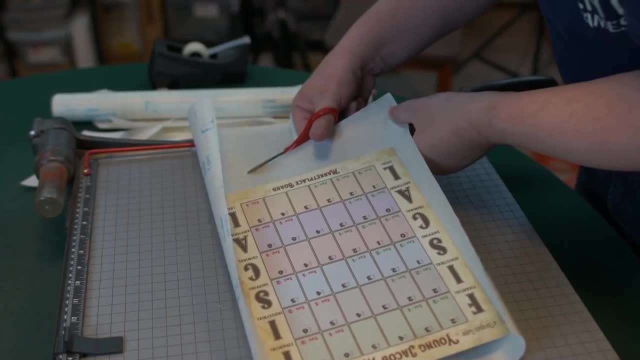 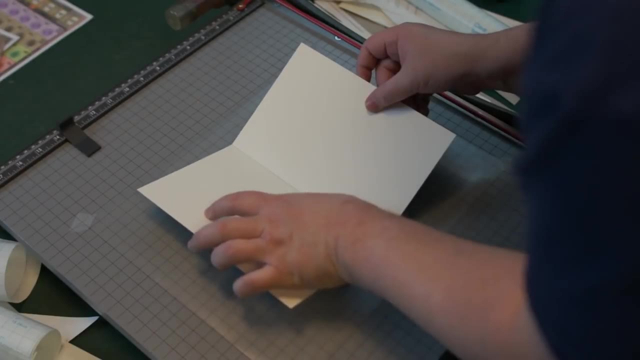 that's about two inches bigger all the way around. I'm using a little bit of scotch tape on the back to hold these board sections together while I stick them to the contact paper, and then that little bit of scotch tape is gonna come off again. 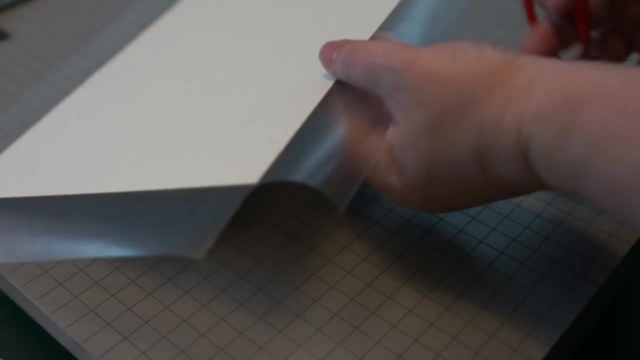 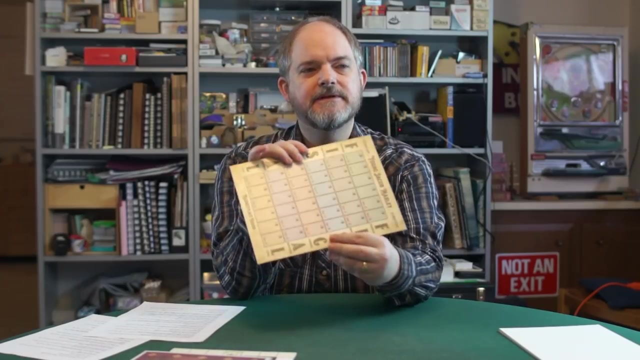 Now I'm cutting out the corners of the contact paper so I can wrap it around the back, and I'm also splitting it at the seam where it's gonna have to break on that fold. And here's the final board with its contact paper Paper hinge. 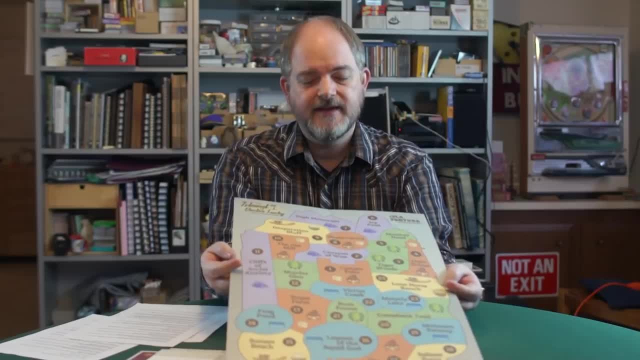 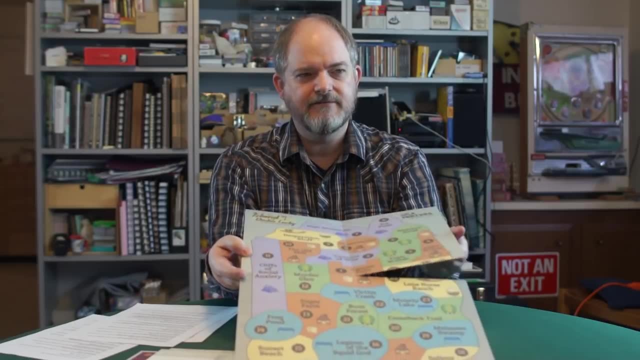 This is a four-piece board. It's a prototype board from the Island of Dr Lucky, and the way we're gonna do this is a forward seam on the top and the bottom and then a back seam on the side, but only on one half of it. 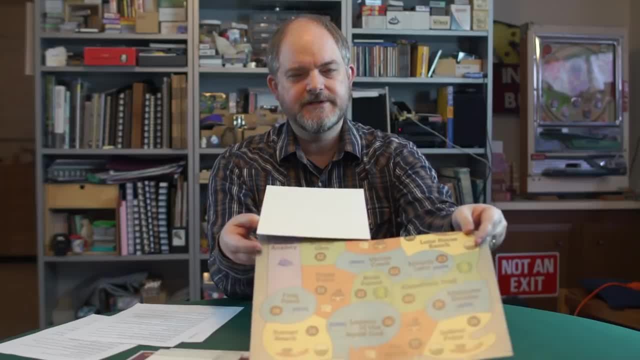 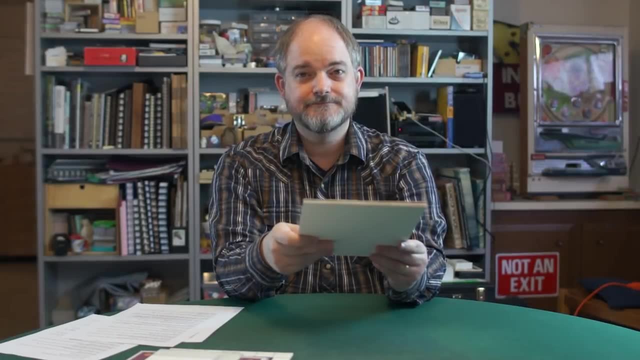 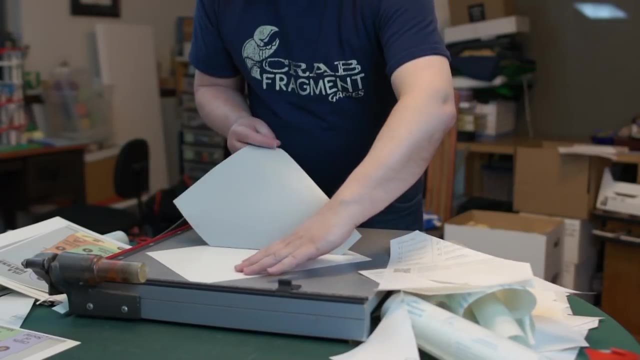 So you see, we've got one open seam here, two forward seams that I've done with contact paper and then a seam on the back with tape that lets it fold into quarters like that. I'm gonna mount each quadrant on a separate board and I'm only gonna trim off the waste. 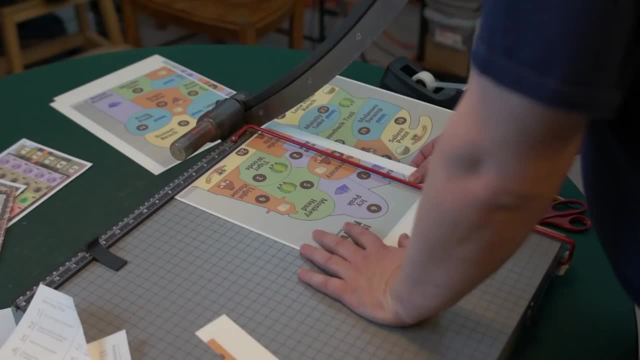 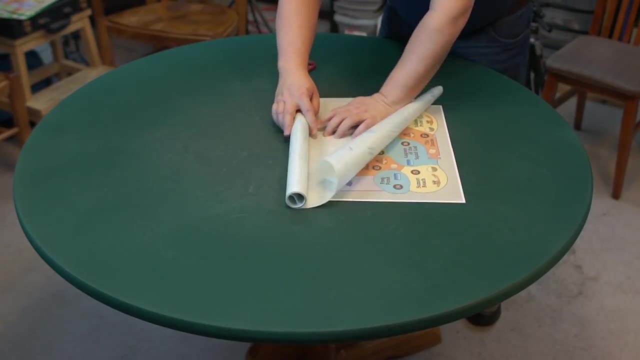 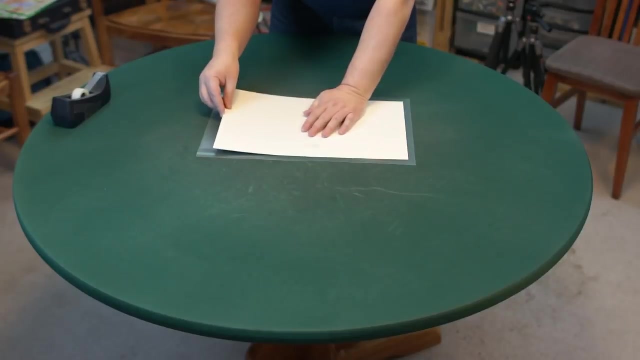 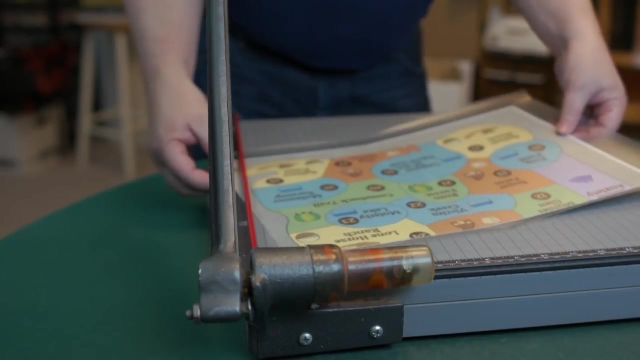 where I need to right before I make a seam. Unlike the Jacob Marley board, I'm not wrapping this, I'm just trimming it off, So the contact paper doesn't wrap around the edges here. but you could do that wrights later. 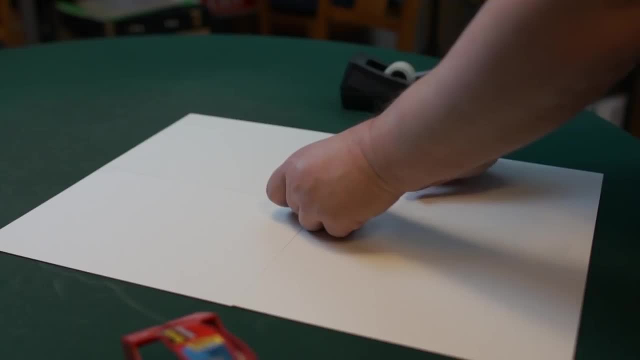 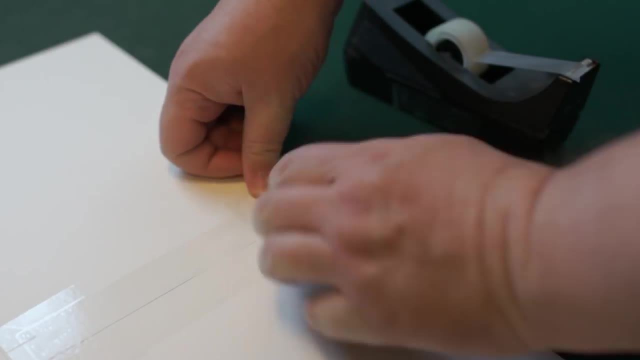 Copying from the other end. if it's a знаете and a posted, you can do it with the wide cut, But for the kicknight shape it's just not gonna be the case here. Keep the center jointhots. 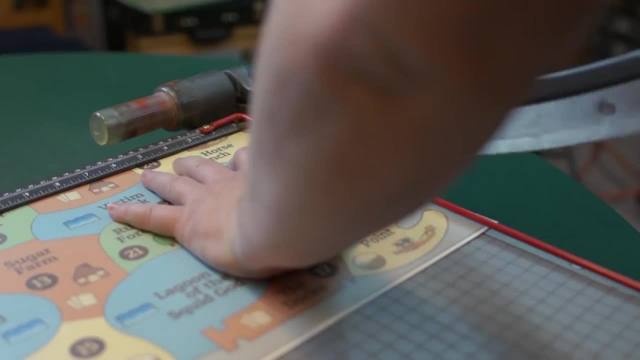 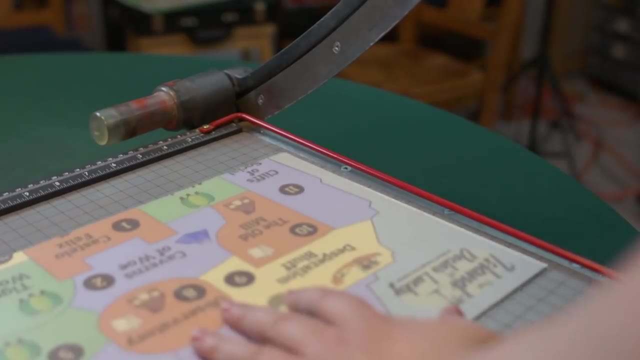 Only tape the bottom ring. they're not gonna be. next, You just tape the sides to halfway through. Don't recommended for the middle seam. And then for the middle seam. I can only tape half of it, but I'm gonna use that same letter: I seam. 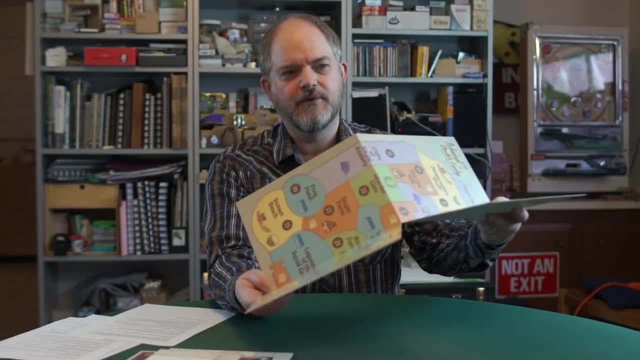 one long piece and 2 cross pieces for a nice sturdy hinge on the palabra on the board that I can tape together. You can make bigger boards with more complicated folds. it's just to alternate between forward and backward seams and they can all compress together like this. 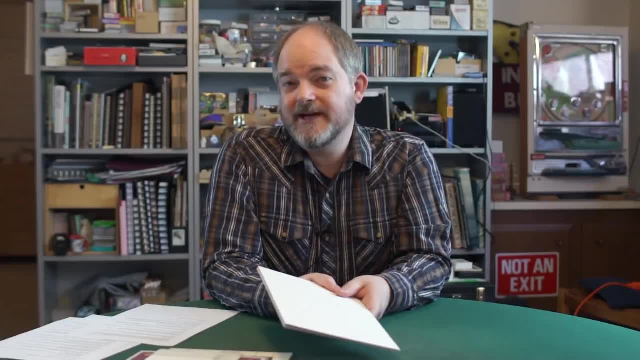 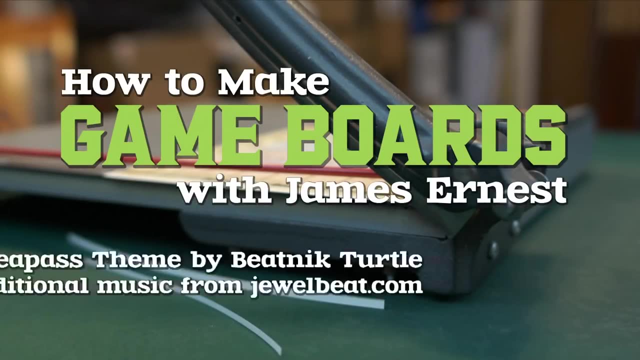 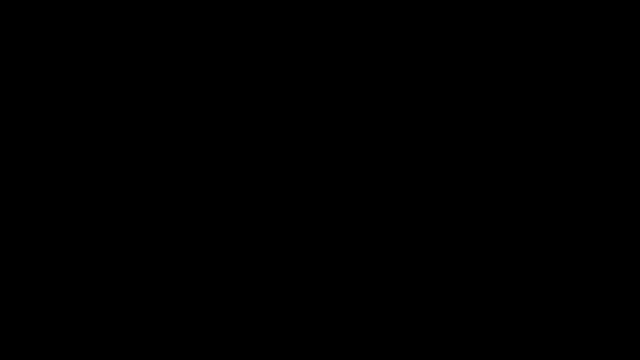 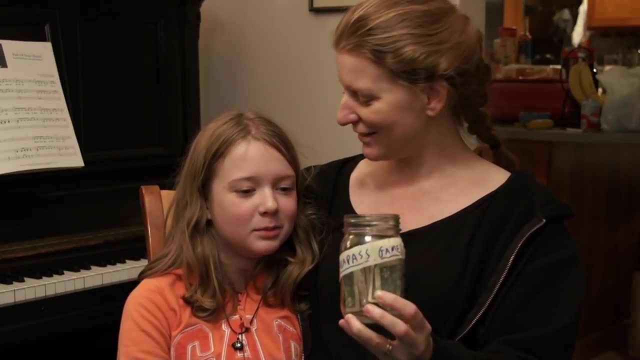 So that's most of the techniques that I use to make prototype game boards. I hope this has been helpful to you and thanks for watching. So what's this? It's a cheap-ass jar. You put money in it and then you send it to CheapAssGames. 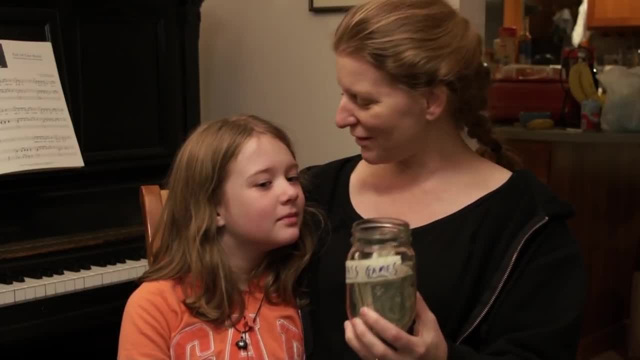 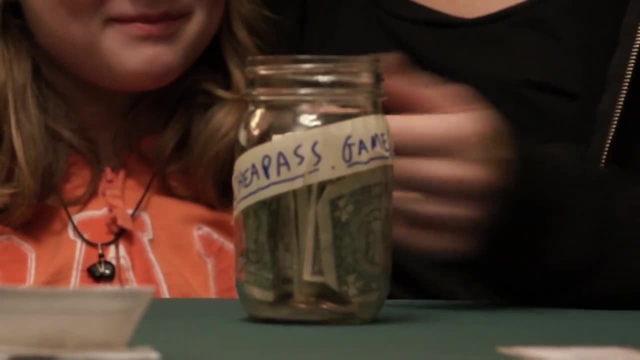 Okay, that makes sense. So you get your friends to come over and play CheapAssGames and if they like them, you put money in the jar and then, when there's enough, you send it in. Makes sense.